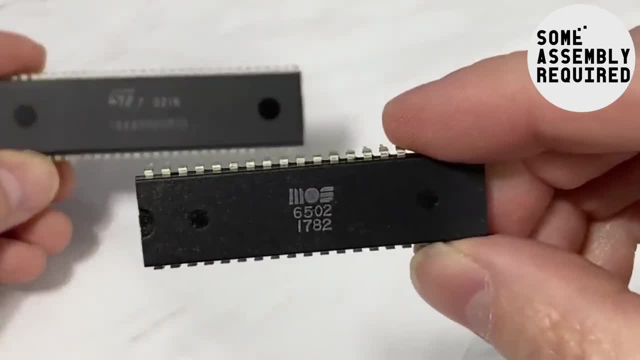 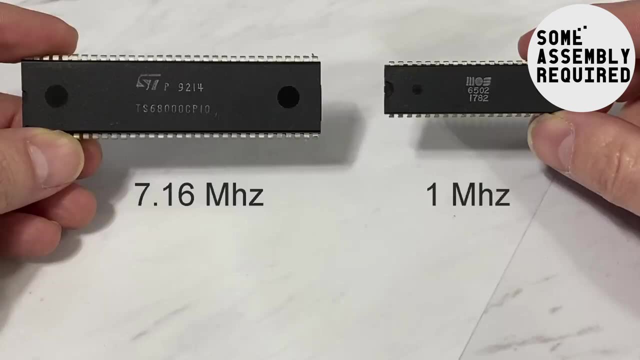 It runs at 7.16 MHz. Now you might think it would be 7 times faster than the CPU in the Commodore 64, which runs at 1 MHz, But that's not actually the case. The 6502 and its variants are very efficient and perform a lot more operations per clock. 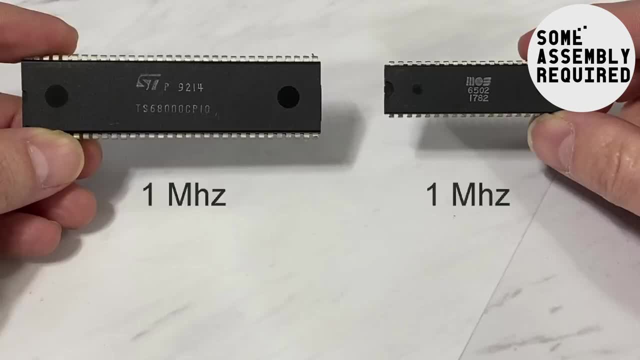 cycle than the 68000.. In fact, if both CPUs were clocked at 1 MHz, the 6502 would achieve 0.43 MIPS, whereas the 68000 would only achieve 0.175 MIPS. But since the 68000 is clocked 7 times faster, it ends up being 1.25 MIPS, which means it's 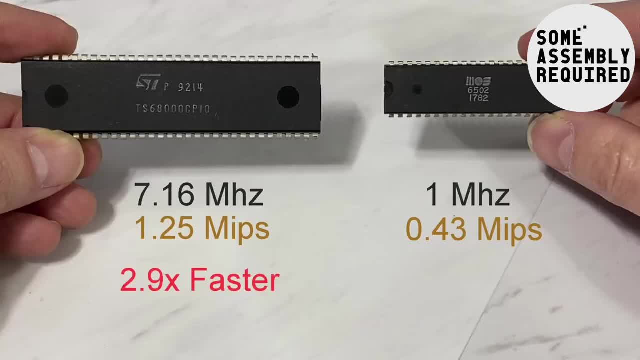 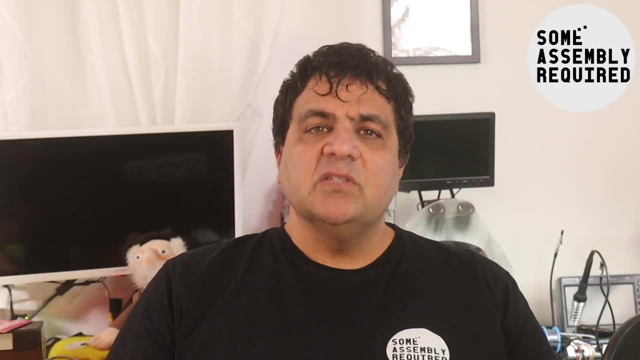 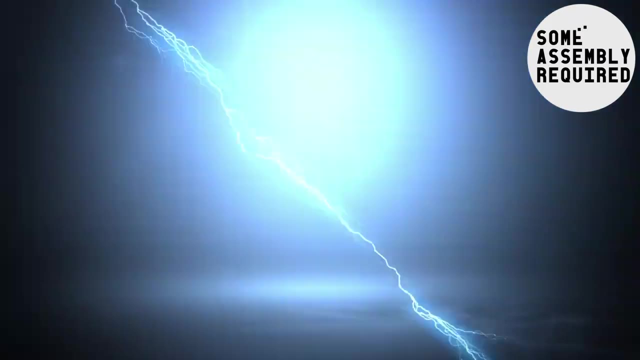 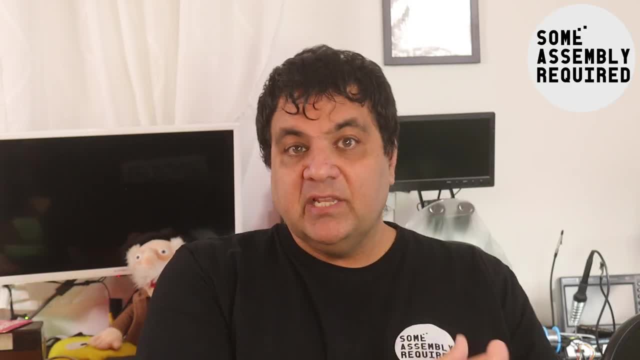 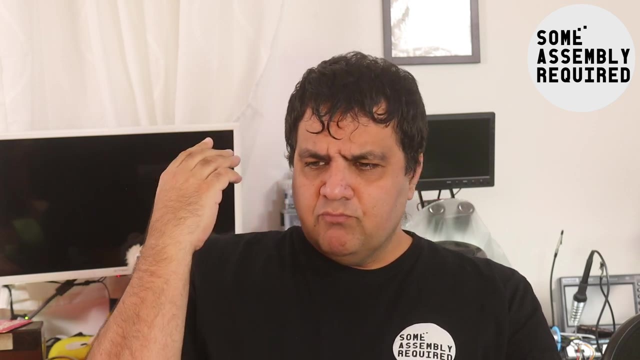 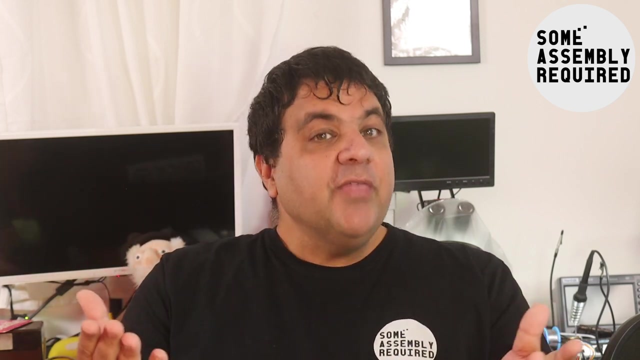 And Ghatis and Apple made a mistake in going with the Apple-Macintosh lines and instead should have gone with Apple 2G. And there he also compares the 68000 that the Macintosh had with the 65816 that the Apple 2GS was going with. 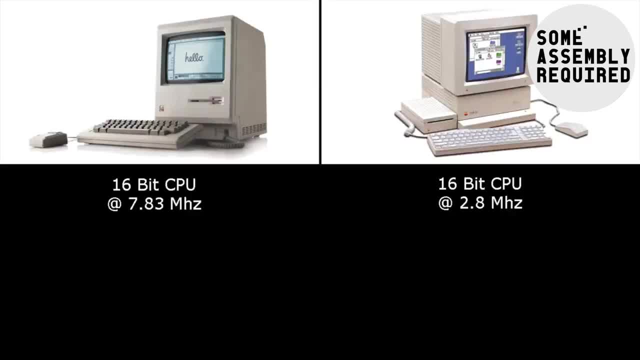 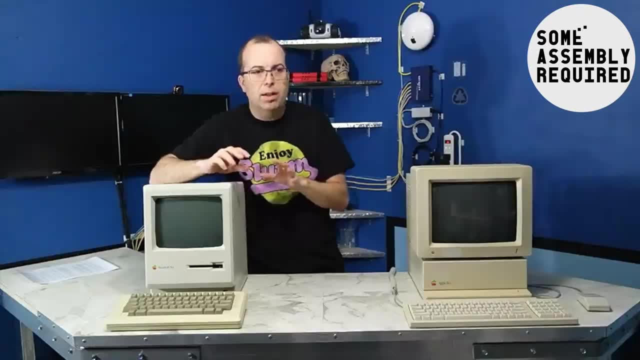 And there he said this: The Mac's CPU had almost 3 times the clock's speed speed. though all right. now what might surprise you is that the motorola chip used in the mac was not as efficient per cycle as the wdc chip used in the apple 2gs. so, as you probably guessed, 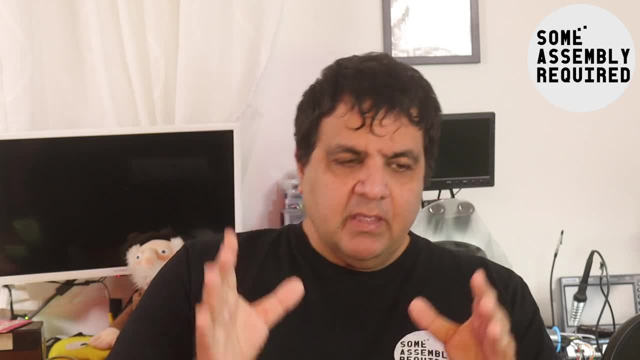 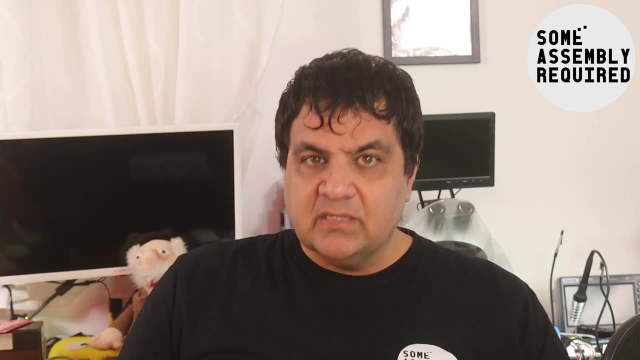 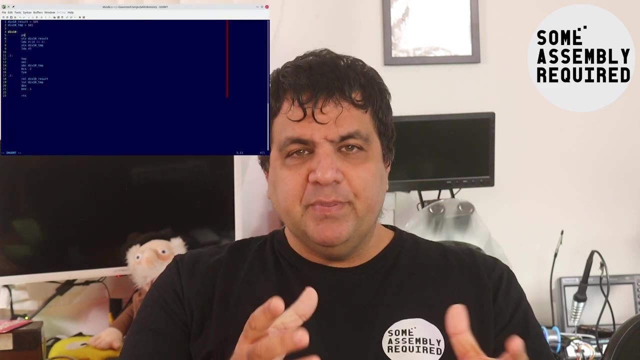 i take issue with this statement. here's the thing now. i did- this isn't the first time i'm bringing this up, in fact, as a response to 8-bit guy's video, um, and the previous time i went really into the weeds and into the details- i built a program that does the same thing for the 6502. 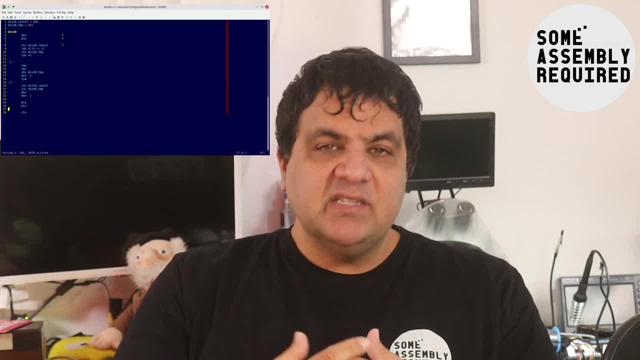 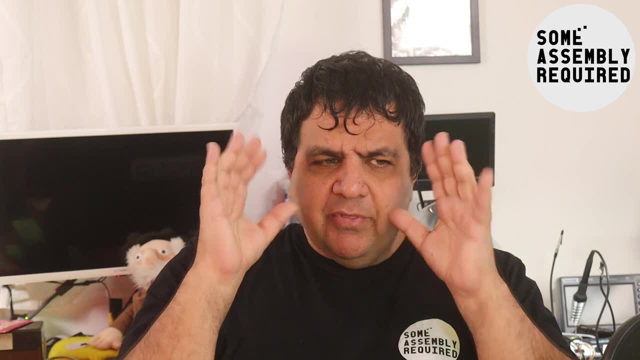 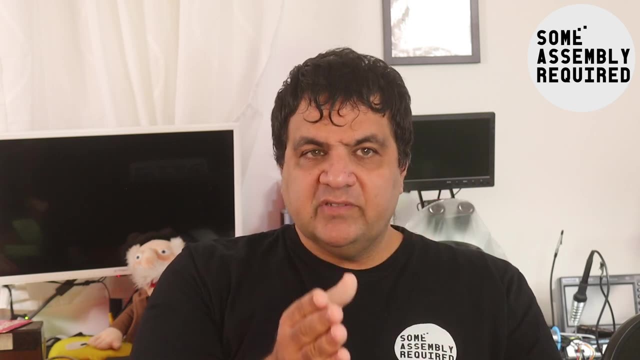 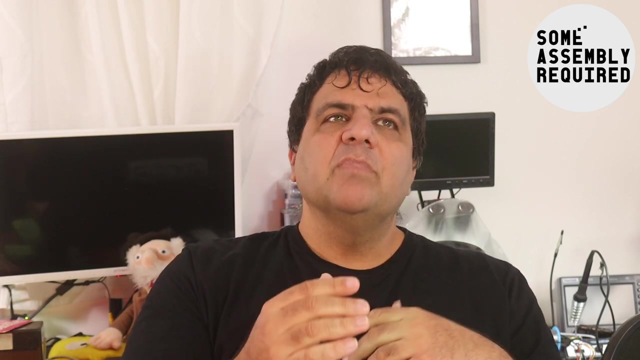 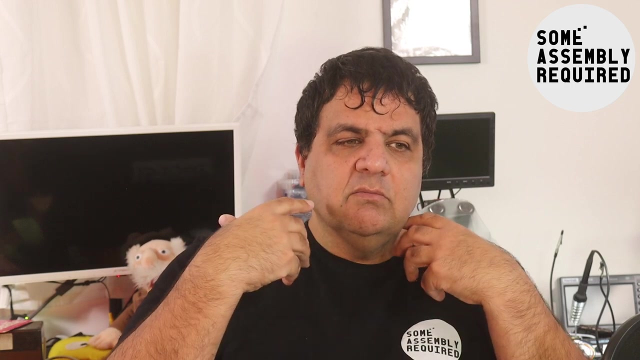 and the motorola 68000 and compared how many cycles each took. if you're interested, check this link. but the the gist of it is this: the 6502 and the csg 4510 which the commodore c65 has is under the same category. i mean it's faster than the 6502, but by around 25. so a typical program. 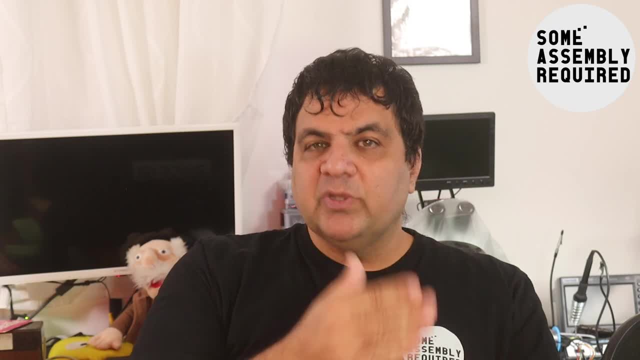 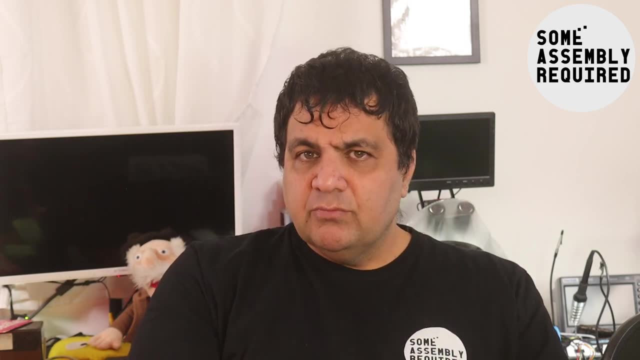 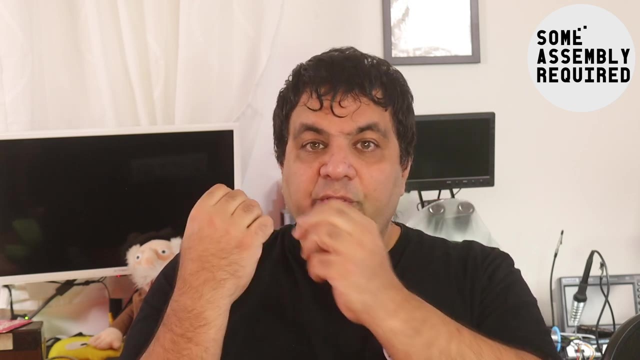 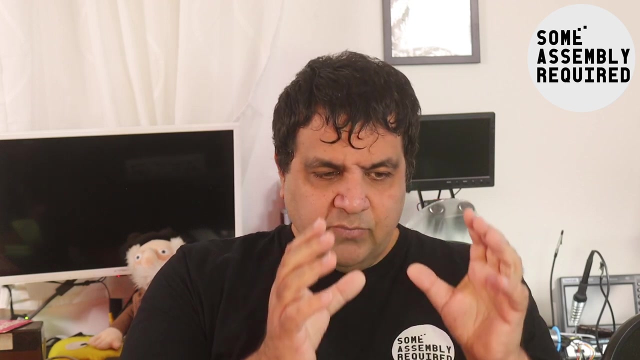 running at the same clock speed will run about 25 faster. however, um, it's still an 8-bit cpu with an 8-bit architecture and an 8-bit bus. the 68000 is a 32-bit architecture cpu with a 16-bit bus, which means that the 6502 is designed to deal with. 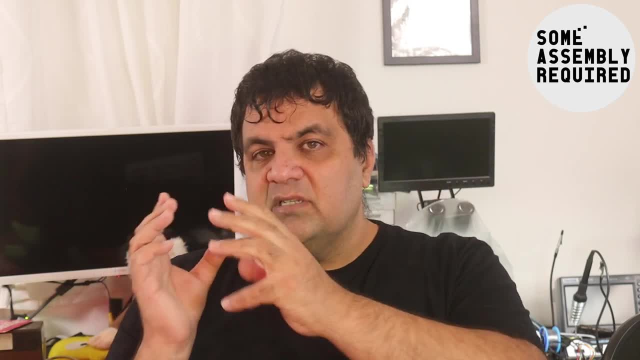 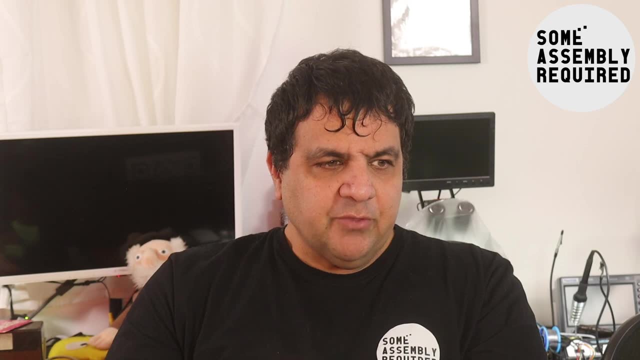 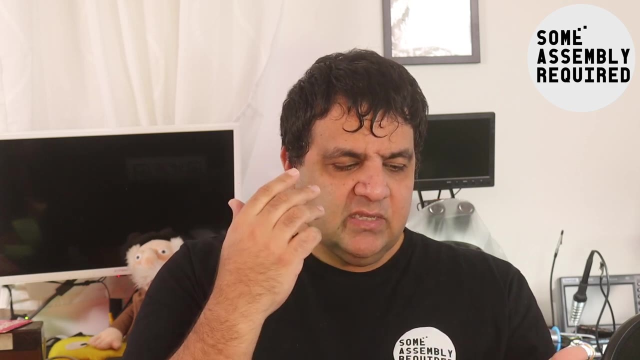 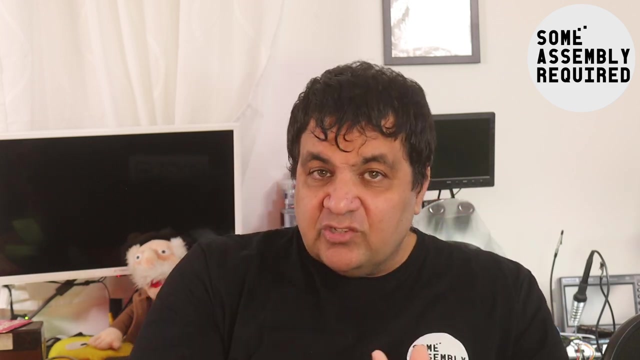 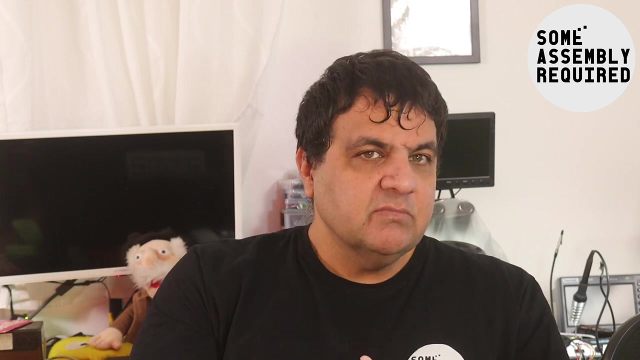 8-bit workloads, whereas the 68000 is designed to be to to handle 32-bit workloads. and if you think about the, the 65816, which um has as a 16-bit architecture with a 24-bit theoretical bus, but actually it's a 16-bit address bus with uh 8-bit data bus. 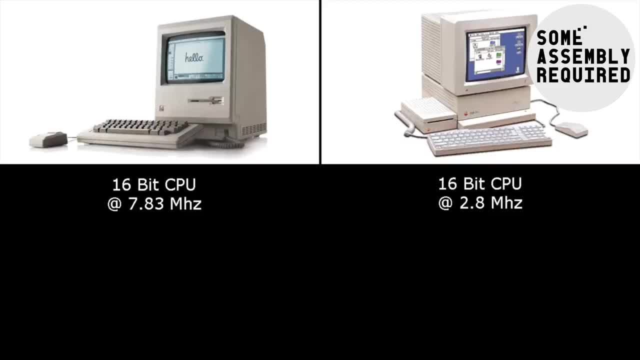 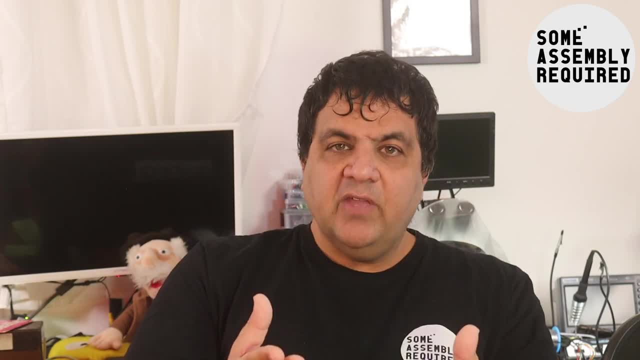 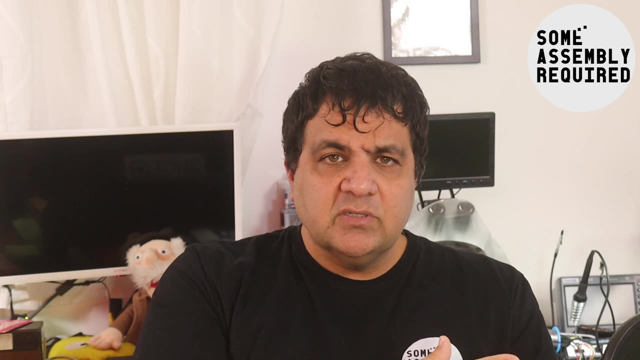 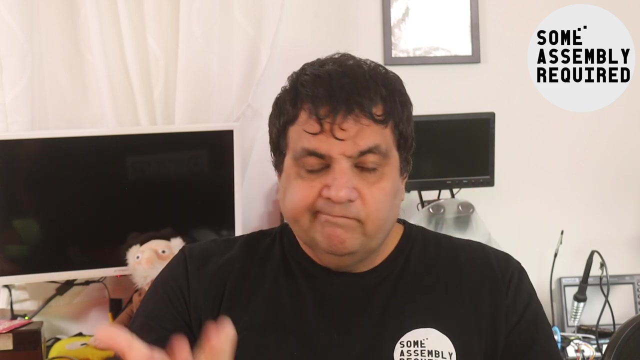 so when david says this, okay, so both machines had a 16-bit cpu- it's just not true. if the 65816 is a 16-bit cpu, then the 68000 is a 32-bit cpu. it's the is a 16-bit CPU, then the 65816 is an 8-bit CPU. It just it doesn't work. Here's the thing. 8-bit workloads mean addresses are known at compile time. bulk transfers are in multiples of 256 bytes and are a single byte at a time. 32-bit workloads are memories dynamically allocated and addresses are from. 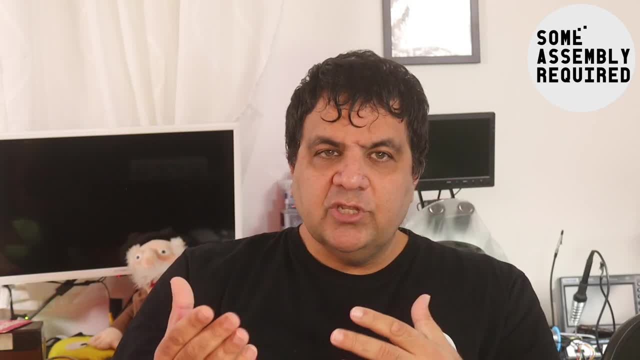 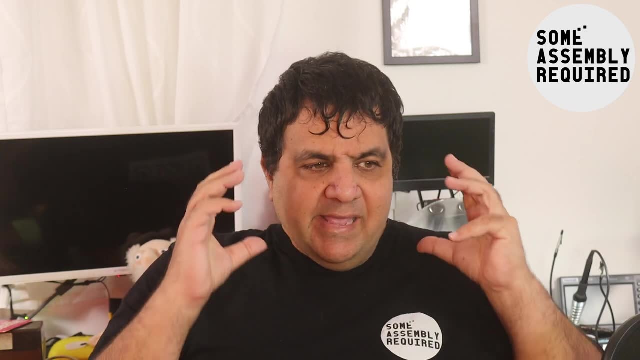 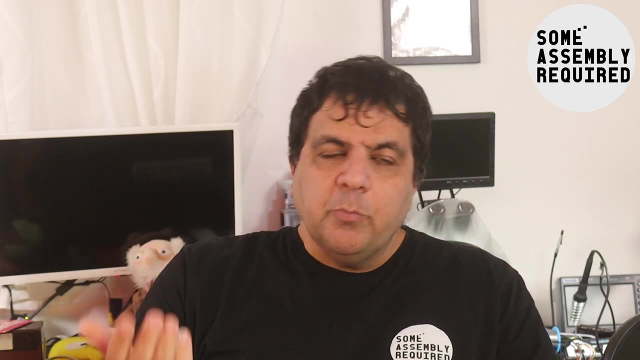 anywhere to anywhere and usually you access them in larger access units, so 16 or 32 bits, And you can't really build multi-process operating system such as the Amiga multitasking, AmigaDOS with the 6502 architecture. with an 8-bit architecture It doesn't. 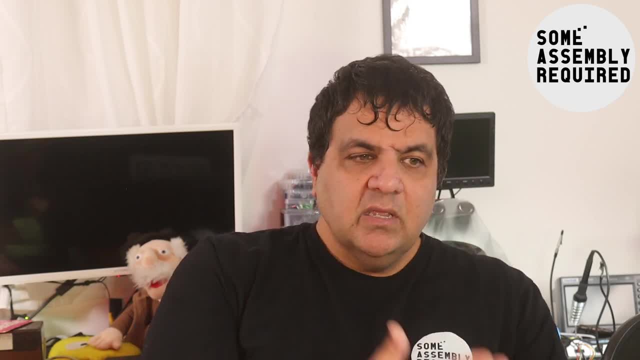 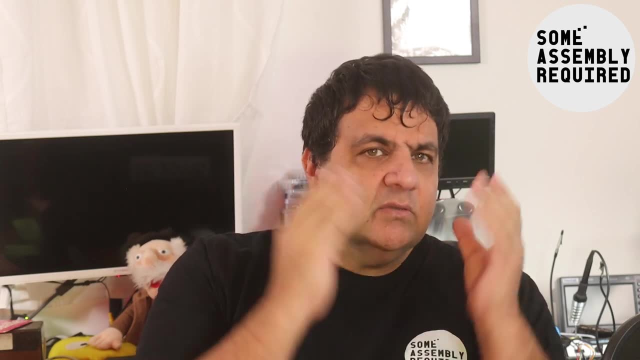 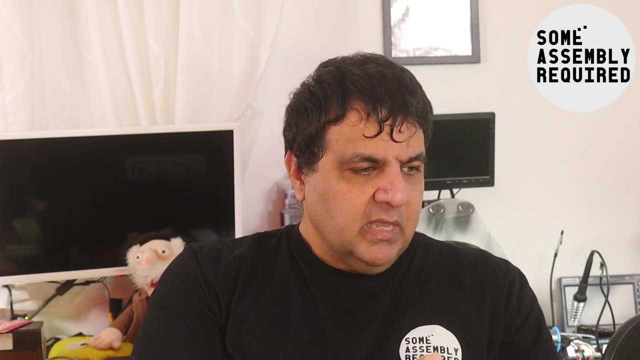 need to be the 6502, it can be the 65816.. The architecture is still 16-bit and still geared toward the 8-bit kind of workloads where addresses are known at compile time. On the other hand, even if you don't go the Amiga route and 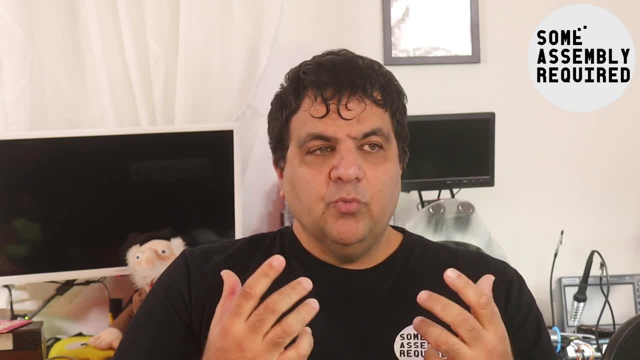 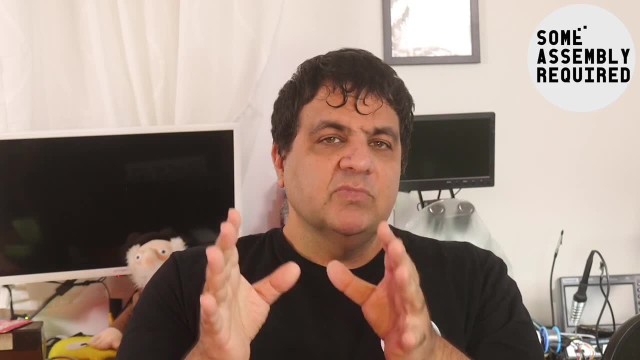 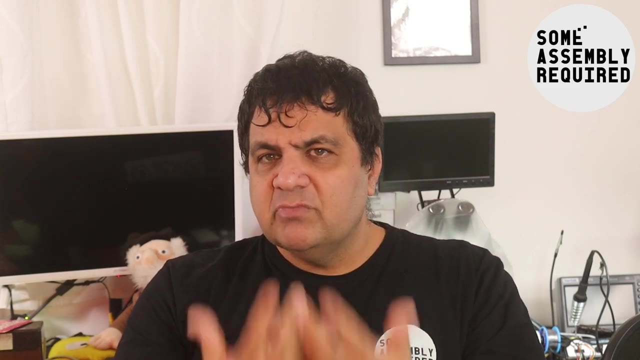 and you ask about the Apple Macintosh, which wasn't multitasking when it was first released. it's still. you could still load several programs into memory, And you can't do that with a 6502-ish architecture. So the idea that the Apple 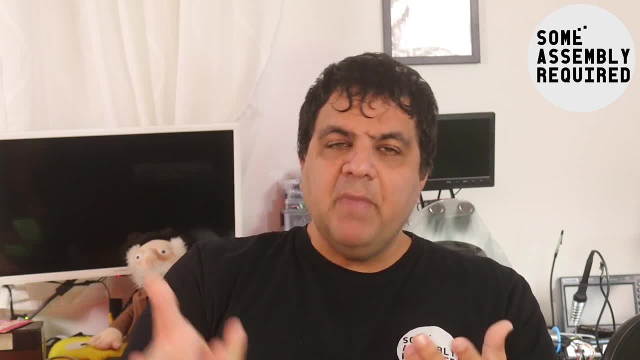 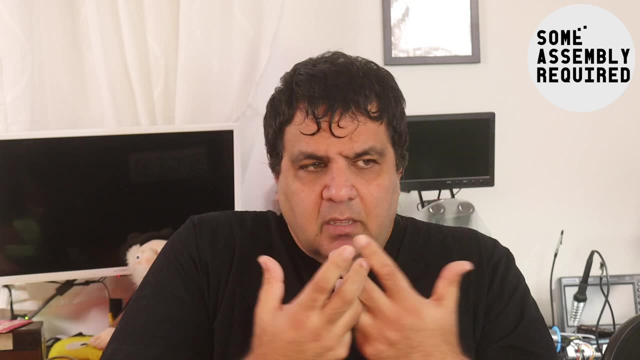 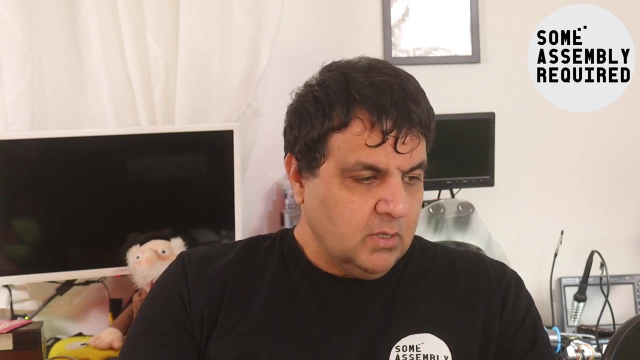 2GS could have replaced the Macintosh, or that the Commodore C65 could replace the Amiga. it just doesn't compute, it doesn't add up, it wasn't possible, it was never possible, And the same goes for the clock. 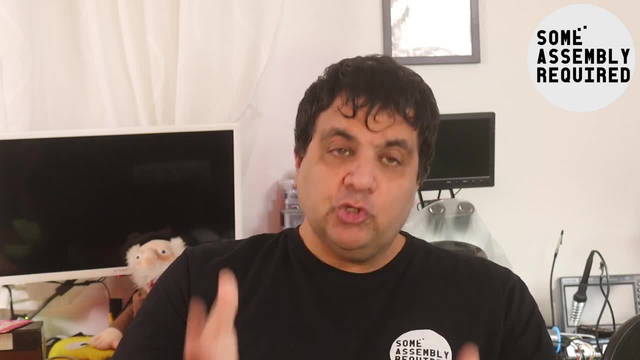 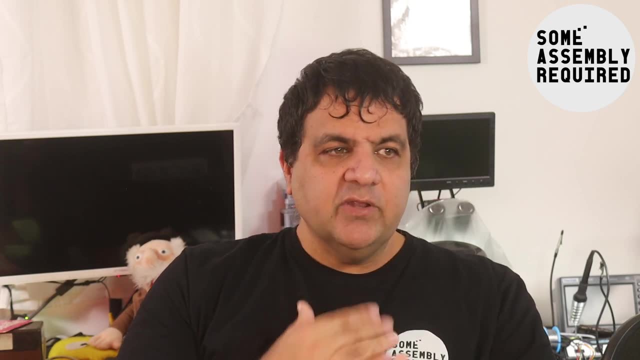 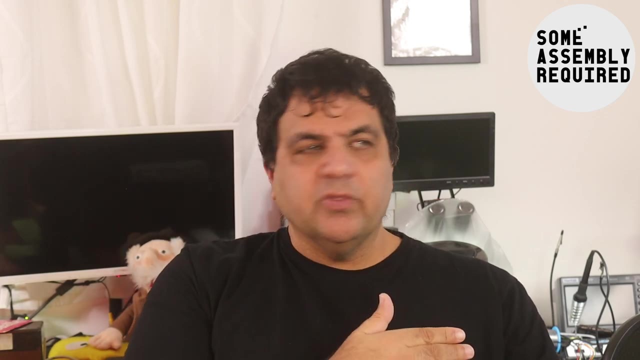 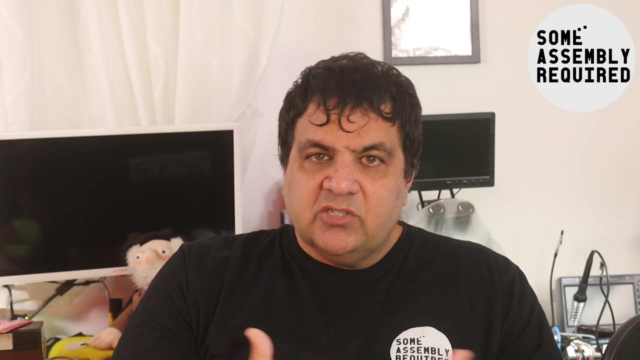 speed. A single instruction, yeah sure, a single instruction. takes less cycles on the 6502, sometimes a lot less and even less, more, even less on the 4510, or the- it was also called the 65CE02.. Sure, a single. 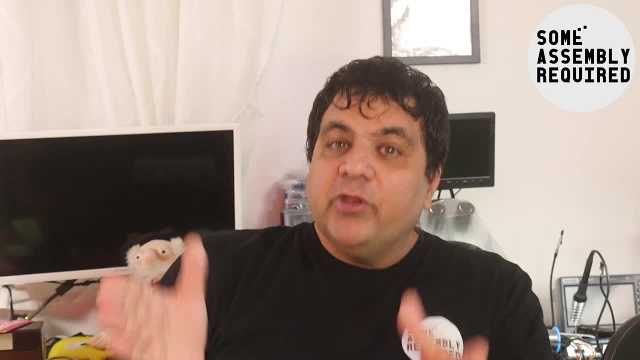 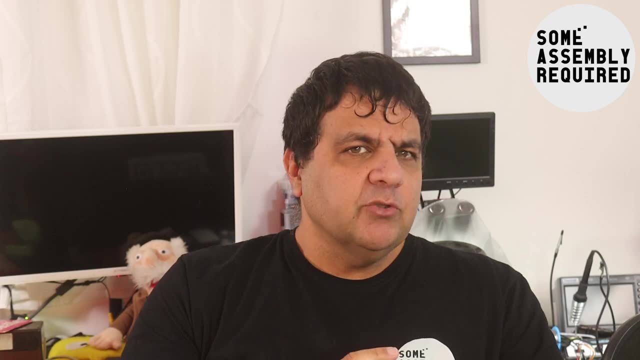 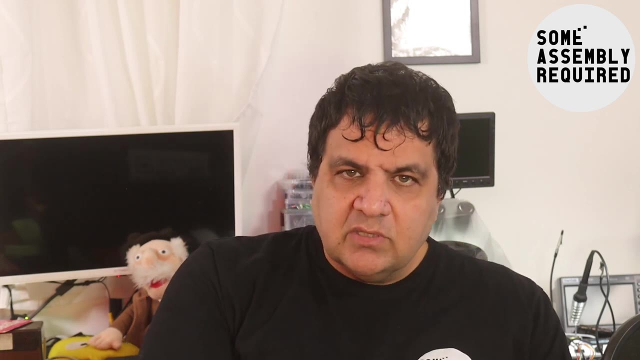 instruction may take less cycles, but a workload, and the thing about my video is that that wasn't a 32-bit workload, that was a 16. an 8-bit workload And still the 68000 did it with less cycles. 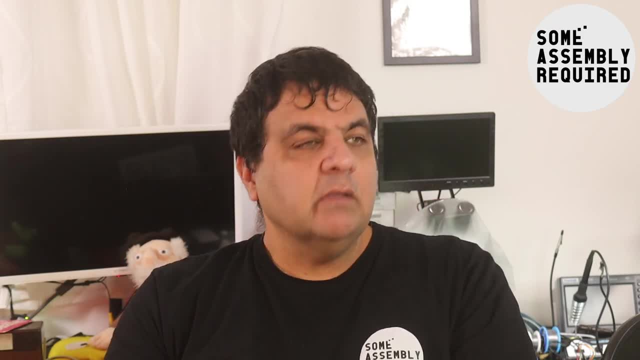 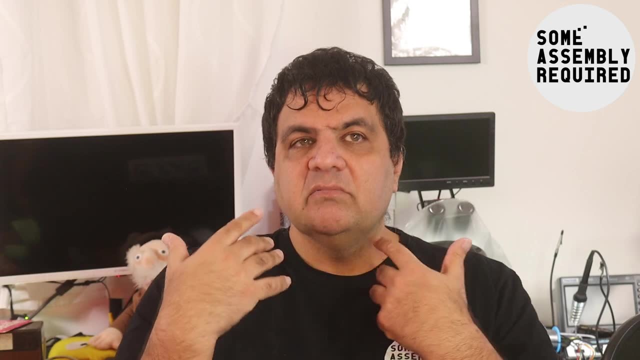 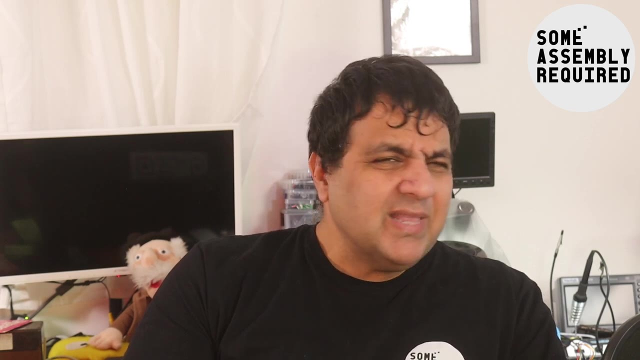 than the 6502.. Now, granted, the 65CE02 may have done it faster, so it wouldn't be. it would be a little faster, but that's still an 8-bit workload. If you go, you just double.